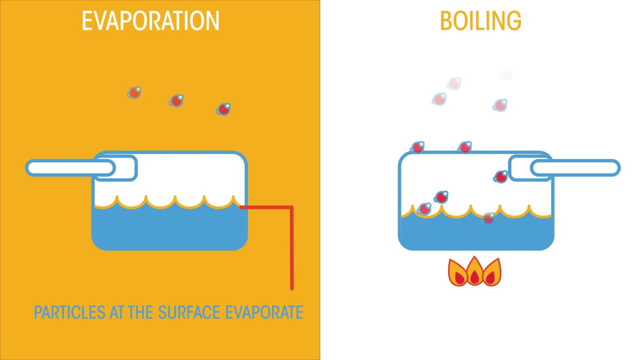 Only the particles at the surface have enough energy to change from a liquid to a gas. Hence evaporation is a slower process than boiling, even though it achieves the same state change. Both are types of vaporization. The opposite of these vaporization. 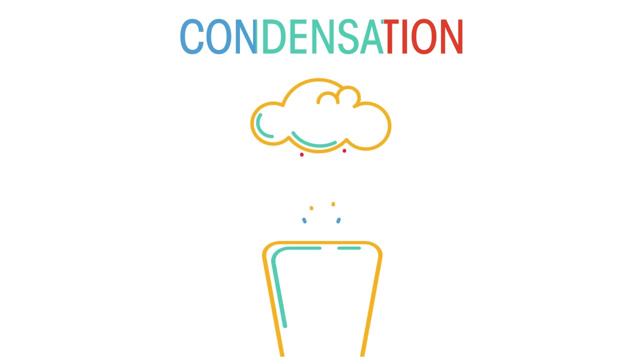 processes is condensation, the transition from a gas to a liquid. Think of a cold can of soda on a hot day, those water droplets on the outsides or the dew on the grass in the morning, or the steamed up mirror after a hot bath, even the clouds in the sky or a foggy windscreen in a 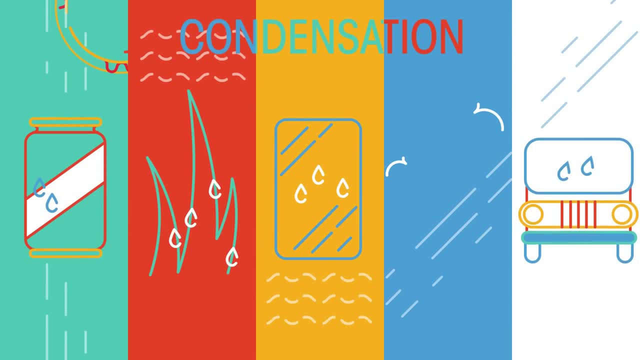 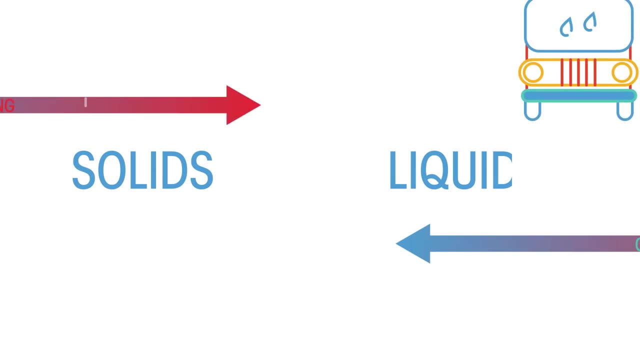 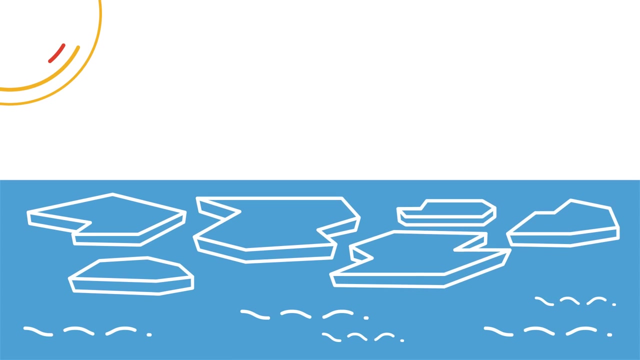 car. These are all examples of condensation. Water vapor in the air has cooled down to form liquid droplets of water. Now let's think about the transitions between solids and liquids, so melting and freezing. Think of the arctic sea ice In the summer, when air temperatures are. 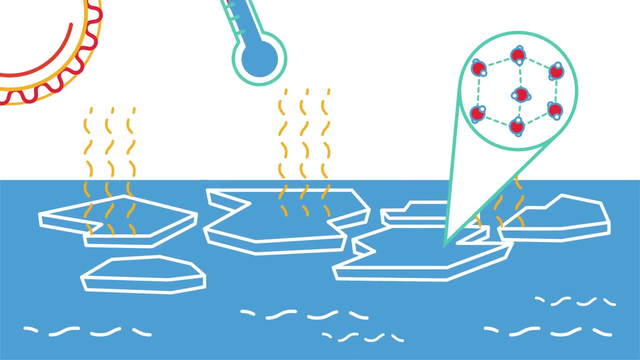 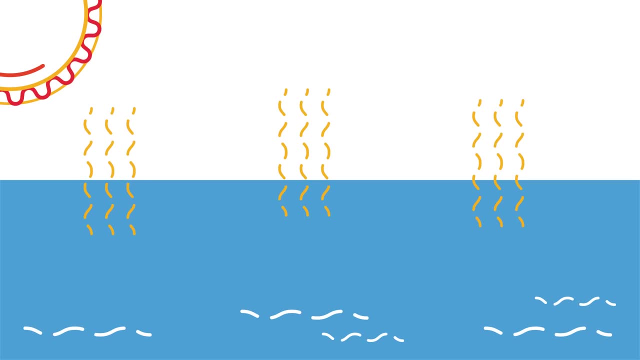 warmer, more heat energy is absorbed by the ice. This causes bonds to break between the ice's water molecules and the ice starts to melt. The solid ice becomes liquid water, But in the winter the air temperatures are colder and so seawater freezes. 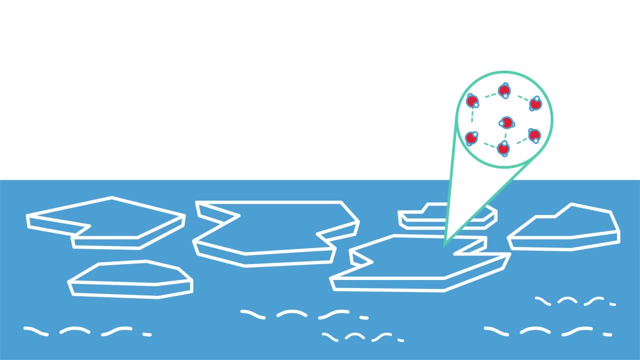 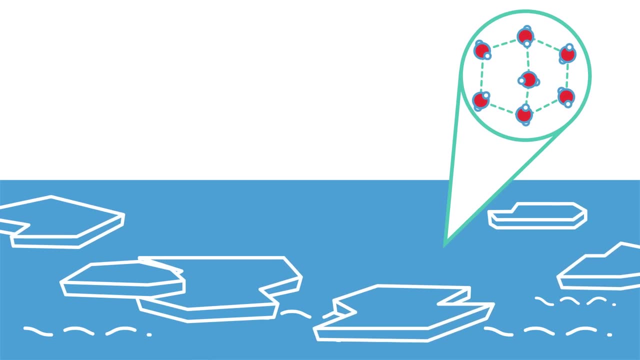 and the ice starts to form again. There is less heat energy within the ice, and so more bonds can form, holding it together as solid ice. So far, so good, But did you know that sometimes, when solids are heated, they can turn straight into liquid? 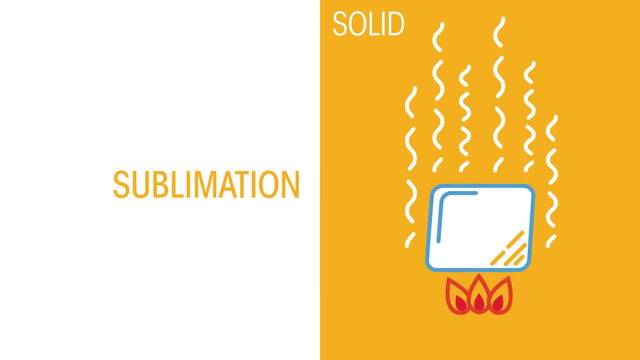 Gases. This is called sublimation. This is only demonstrated by particular materials such as solid carbon dioxide, also known as dry ice. When subjected to a certain pressure, it will turn straight into gaseous carbon dioxide. Liquid carbon dioxide does exist, but it only occurs. 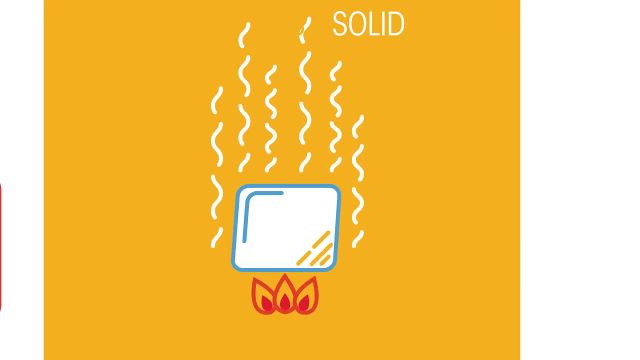 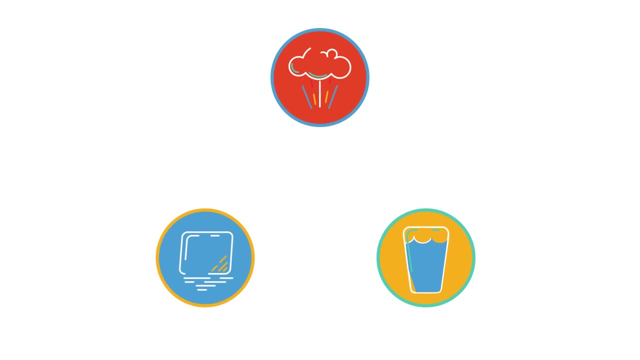 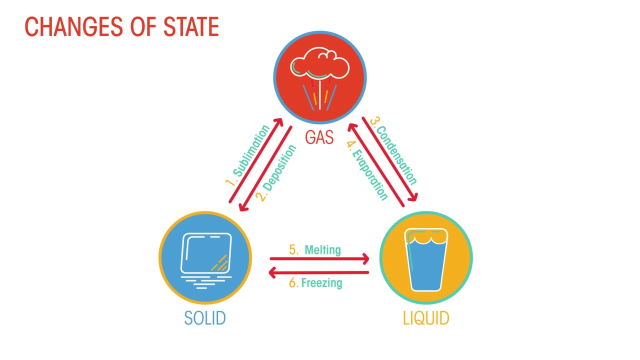 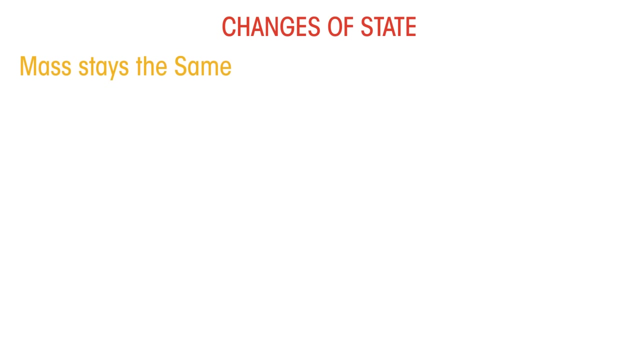 under very high pressures. Similarly, gases can turn straight into solids when cooled. This is called deposition. Let's check out how much you remember about the changes of state. Pause the video and fill in the blanks. Did you remember them all? Our final thing to discover is that when a material changes states, the mass stays the same.